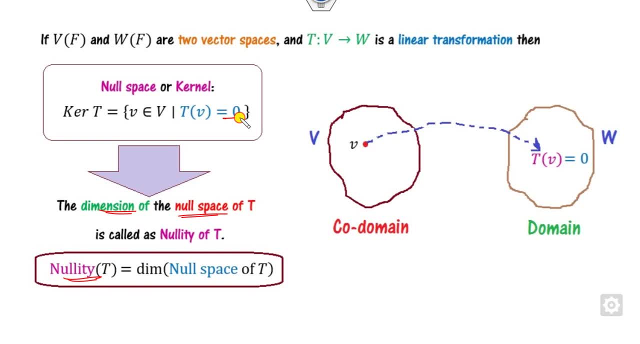 nullity of the null space. That's why it's called as null space, because it goes to the zero. So, for example, here this: how many elements, such kind of the elements are there? we will call as the nullity of this. 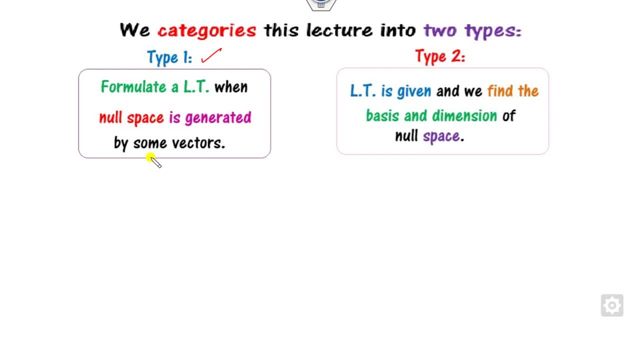 So how you can find that? we will discretize this into the two categories. First one is you have to formulate the linear transformation whose null space is given to you. Second thing is when linear transformation is given to you and you have to find the null space that is a. both are vice versa. 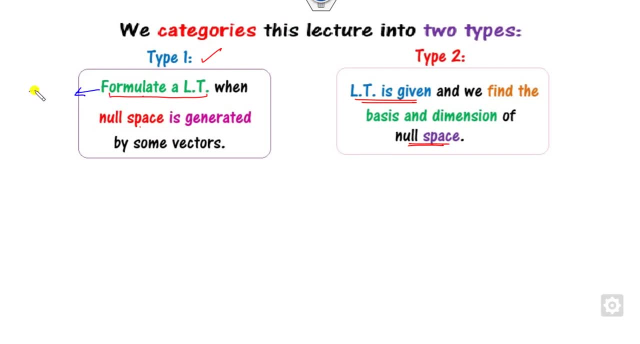 are there, In this case, the linear transformation. your target is to formulate the null linear transformation and the null space is given to you, While in this case, the linear transformation is given to you and your target is to find the null space. For example, 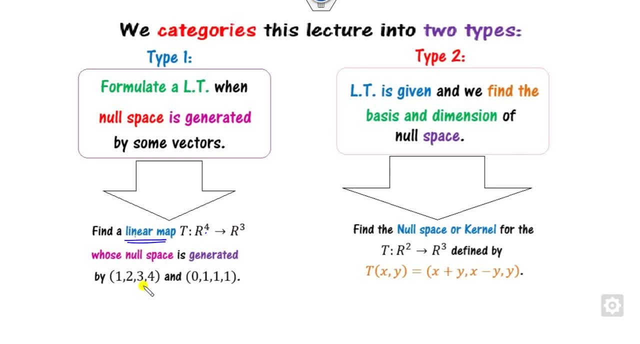 here you can see, your target is to find the linear transformation, whose null space is here. Second one is: you have to find the null space with linear transformation. is here how you can solve this kind of the problem. So, firstly, before we start, firstly, you should remember that kernel of 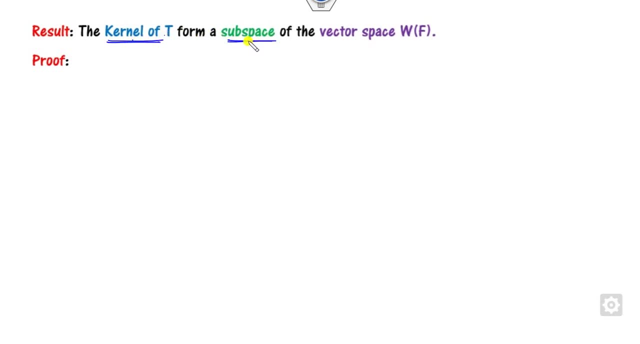 this vector space always be a subspace of this. how you can prove that? that's a very simple. firstly, you have to write the definition of the kernel, like here. how you can prove the subspace, that is, you have to take the two elements, v1 and v2.. 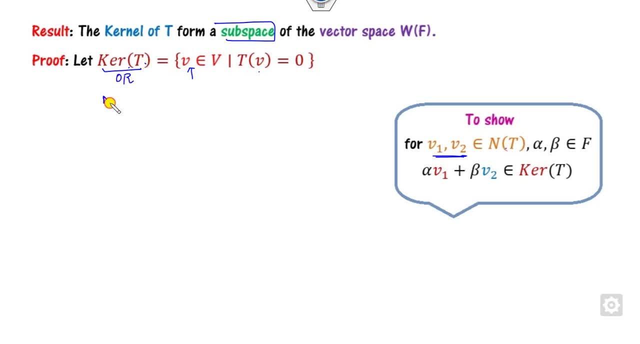 So v1 is the kernel or n of t. this is kernel, or called as null. this is same. elements are there, then you have to prove that the linear combination will also be there. That's a very simple. we can start with the once v1 and v2. here it means this condition satisfied. Now you can take, since kernel is the, 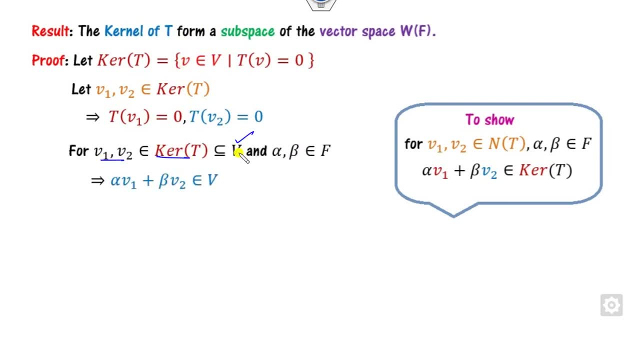 subset of the vector space. So it means v1 and v2 are also belongs to the V, and alpha and beta is the field. So therefore the linear combination is there because v is my vector space. So once v is a vector space, the closer property holds me. Now your target is to prove this value as my zero. how you can? 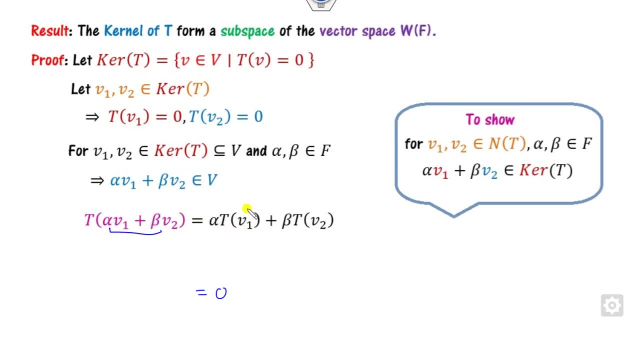 prove that. I can start from here. because t is linear. I can open this. what is the value of that t? v1, this is zero. this value is also be zero, so it is a zero. So if the mapping is zero, it means this: 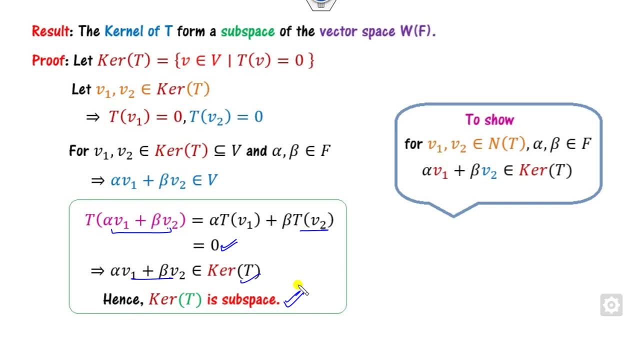 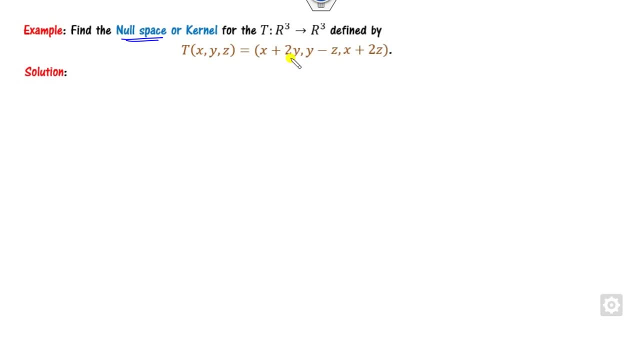 belongs to the kernel, hence it's a subspace. Now look at that. the first step is when you have to find the null space or the kernel. when transformation is given to you, The kernel or the nullity is my here, So we can substitute the value of the v. v is my x, y, z Here. what will? 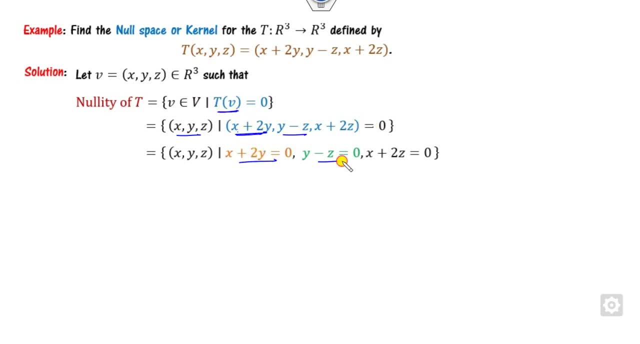 happen. if t is zero, it means the first component is zero, second component is zero, third component is zero. Now your target is to find the value of the x, y and z. Now clearly sees that. from here, what is the value of? 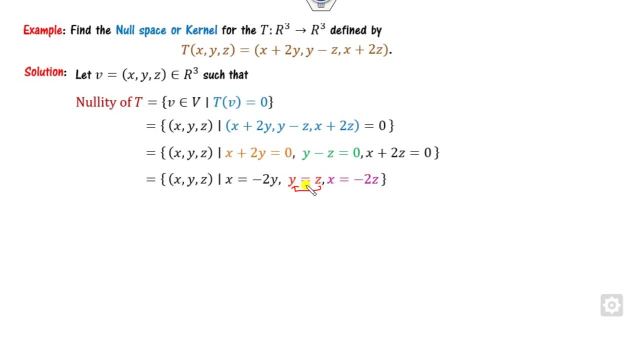 the y. y is nothing but my z. From here I can find the value of the x. from here I can find Now, since y is equal to z. so and both the values here, look at that x is equal to two z, x is equal to two y, So we can equate them. we can see both are. 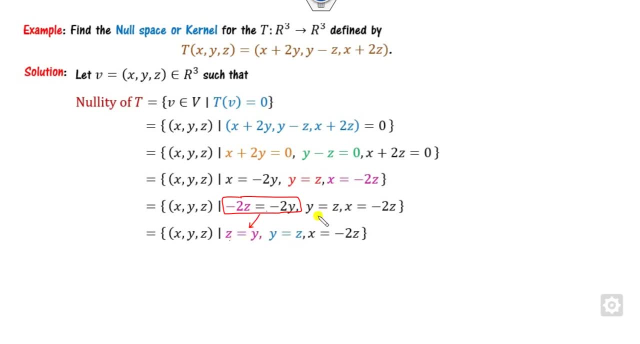 equal, and after the solution we will get y, z is y, y is equal to z, and so on. Now I can substitute all the values. add here: what is the value of the x? x is my minus of two, z, x is my minus of two, z. y is equal to z and z is. 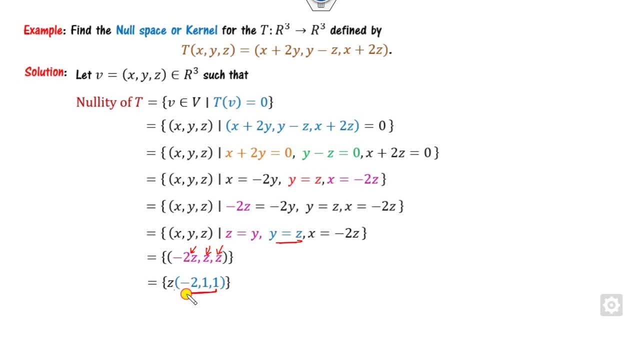 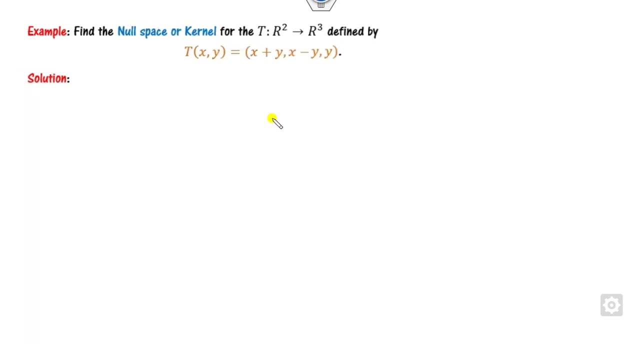 equal to z, So I can take z as a common and here so, since this is the one element and the rest of them the scalar multiplier of this, So we can see this form, a basis, and the nullity, and how many elements are there? Only one, So that is why the nullity is my 1.. Look at the one more example. 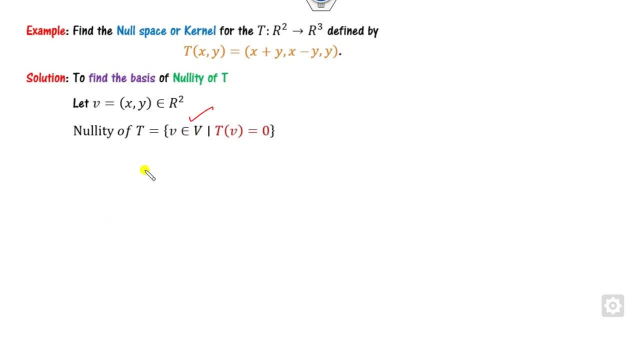 out there Again. transformation is given to you. We can start from here Now, since these are the elements of the R2, so I can take this as a R2 elements. So what is the meaning of that? It means x plus y is equal to 0, x minus y is equal to 0 and y is equal to 0. So we can solve them. 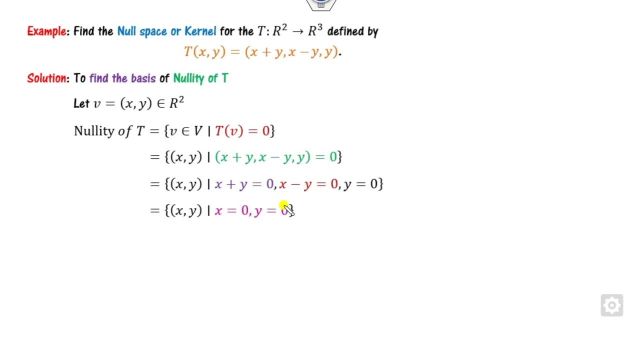 Once you will solve this value. what is the answer of this? You can see, y is equal to 0. if you substitute here, x is 0 and here. So if you substitute this value, this means that is only for the nullity. that is a 0 element. It means the nullity is my 0.. Look at the second case. 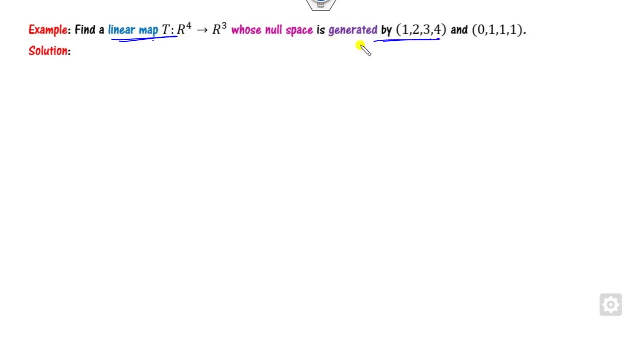 when you have to formulate the linear transformation, when null space is given to you, what is actually given to you, That is, by the definition of the null spaces. T of this element will goes to the 0,. T of this element will goes to the 0,. 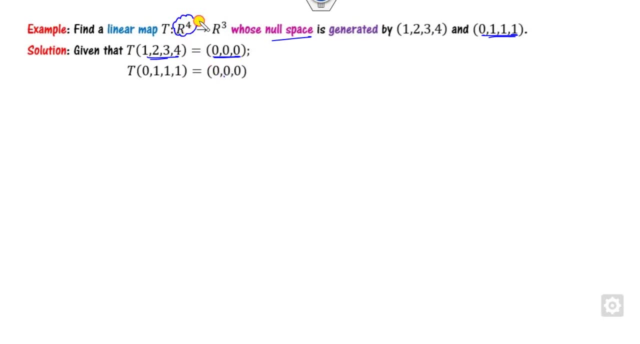 T of this element will goes to the 0, element will goes to the zero and since the core domain is my r4, it means the two elements are there. our target is to find two more elements so that it will become becomes the four elements are. 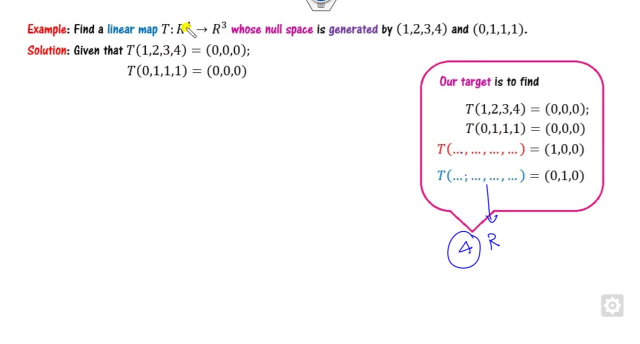 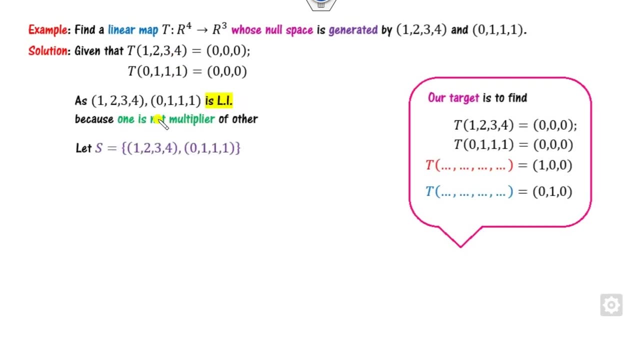 there. if it is a r cube, then we will see in the next example. if it is r cube, then there is only need of the one element now, how you can find these two elements. so that's very simple. so firstly, you have to check whether these two elements, whatever the given to you, they are linear, independent or 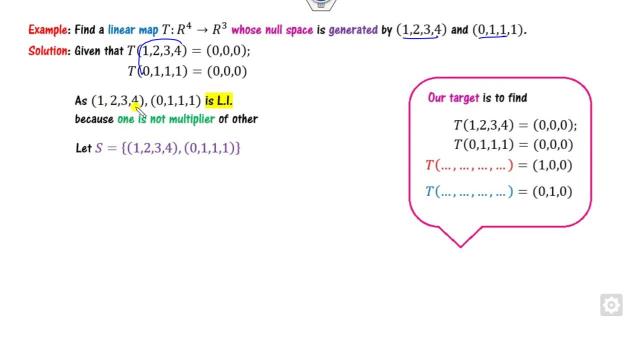 dependent clearly see that one cannot be written as the scalar multiple of the others, because you can see, if you divide it by two, it becomes a one, that's two, but it will not be there. it means this is not the scalar multiple. so once if they are ally, you can consider, as here, what are the standard. 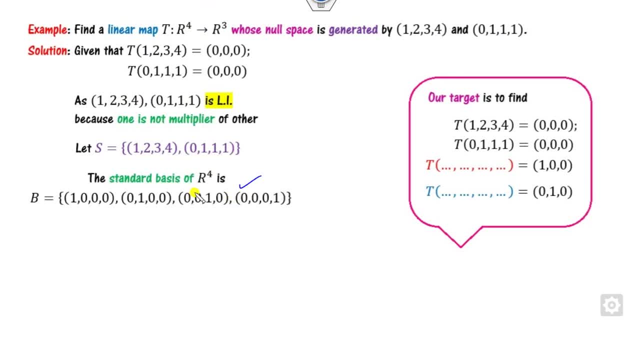 basis of the r4. these are the my standard basis of r4. now you can combine both the basis as union b now, since we need the two elements. so out of these six you have to find the two elements. how you can formulate these two elements from here. you can formulate the matrix, always here. that is first, element one, two and we. 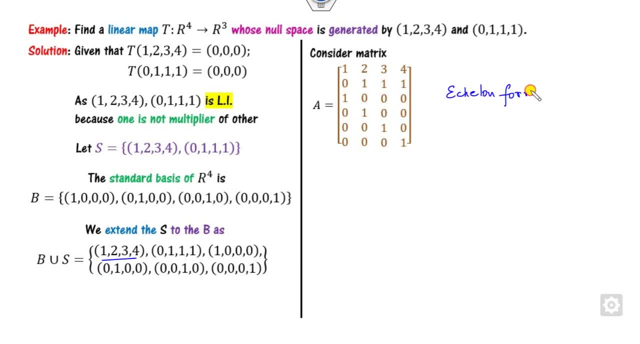 will try to convert into the echelon form. once you will find into the echelon form by using the row operations r2 minus r1, r3 minus r1 and so on. the rest of one will be a here. so your first target is to come this value as a zero by using this operation. 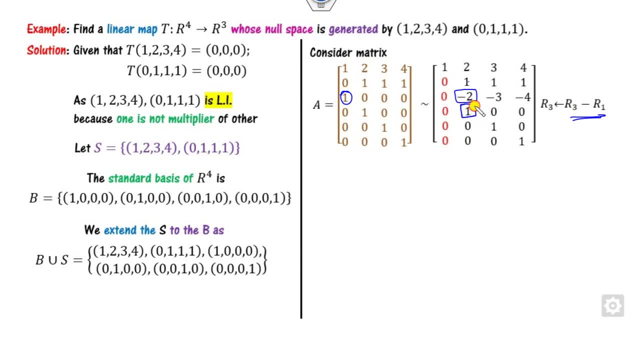 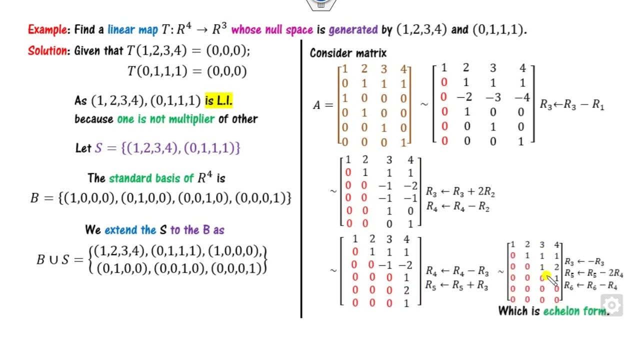 now you can make this value as a zero. twice of this. you can make this value as a zero by using this operations. now you can make them- this value as a zero, this value as a zero, by using the row operations like of here. now your target is to make these two values as a zero by using here. 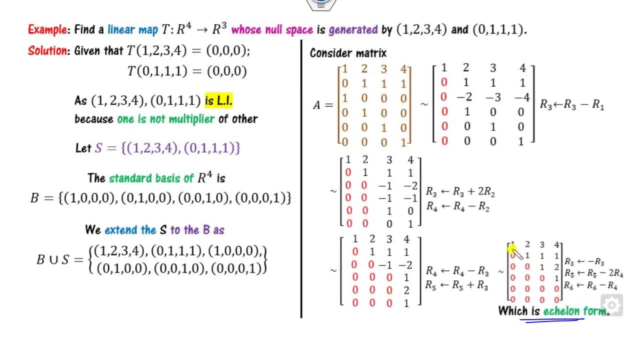 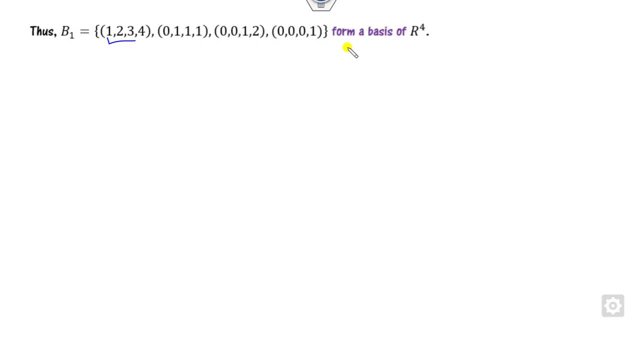 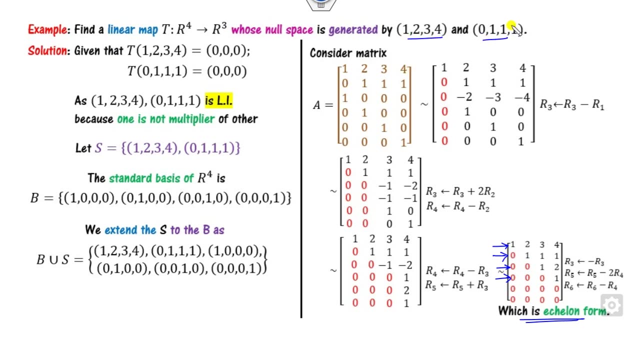 now clearly sees that these are my echelon forms. so how many rows are there? they are no zero. these are the first four elements. are the four rows, so i can write this value as here, this for my basis, and you will be see that the first two elements are always be given as of this one. so we need the. 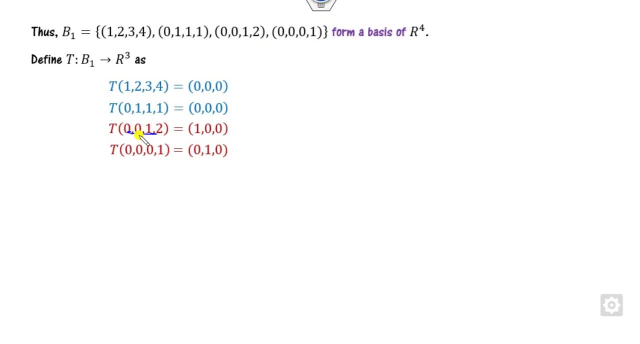 two more elements that will be here. you can see, this value is my here. this value is my now. once you will formulate this value, we can take any of the elements from the r4, because they are the four element we can write here. our target is to find the value of the alpha 1, alpha 2, alpha 3 and alpha. 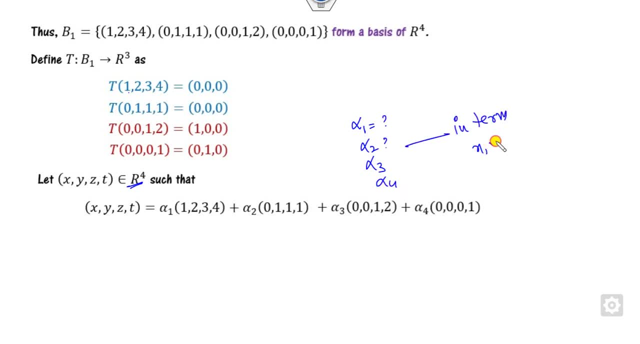 4 in terms of x, y, z and t. if you are able to find this, then you will be able to find the value of the matrix. then we can proceed them. you can equally the coefficients. now, from here you can see. alpha one is my x. i can substitute this alpha 1. here can you find the value of the alpha 2? you can easily. 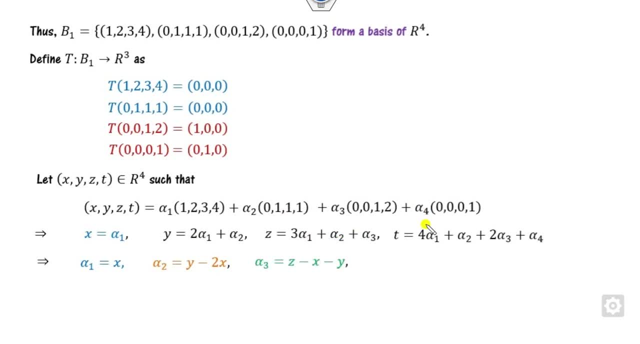 find. i can substitute this: alpha 1 and alpha 2. here we can find the value of the alpha 3. i can substitute alpha 1, alpha 2 and alpha 3. here we can find the value of alpha 4. now, since all the values are in terms of the xyz, we can substitute here. we will get this here now. apply the transmit. 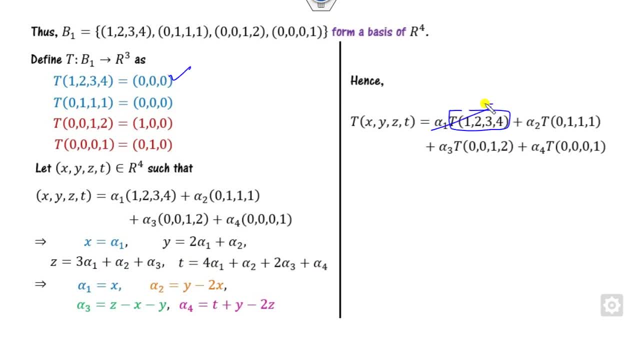 is the value of this? this value is my 0, so there is no need to write. this value is also be a 0. this value is my 1 0, 0 and value of the alpha 3 is my here value of alpha 4. is this now after? 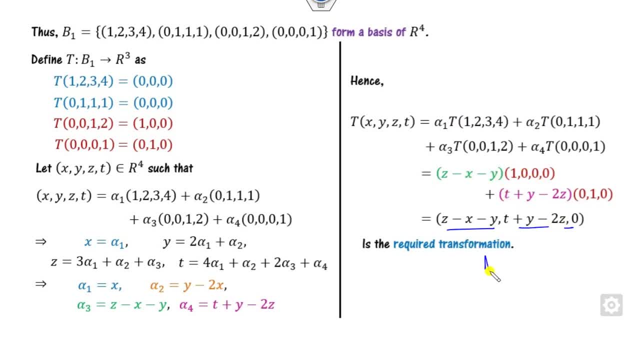 solving it. you can open this, you will get this as a linear transformation and you can subject that. whether your answer is correct or not, you can verify it, whether this will satisfy it or not. look at one more example, are there? so, again, the null space is given to you. 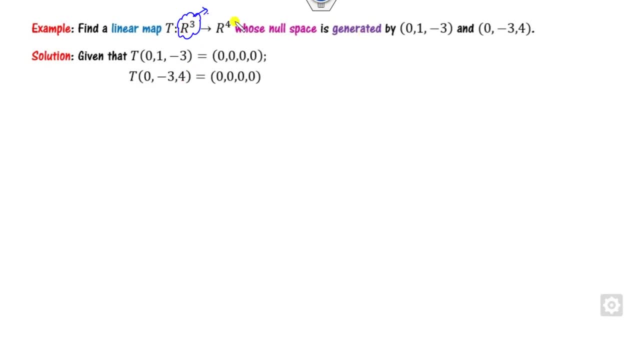 in this case, these are my r cube, so you can see the two elements are given to you. it means your target is to find the only one element. how you can find that? that is a very simple. firstly, you have to check whether they are ally. you can clearly see again, since it is a r cube, so you 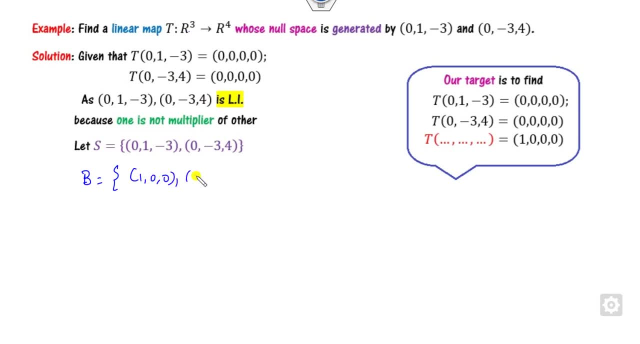 can consider as a standard basis: 1 0, 0, 0, 1 0 and 0 0 1 are there and write the b union s collection of all those elements. write the matrix a. otherwise what you can do is you have to think one value in such a way that 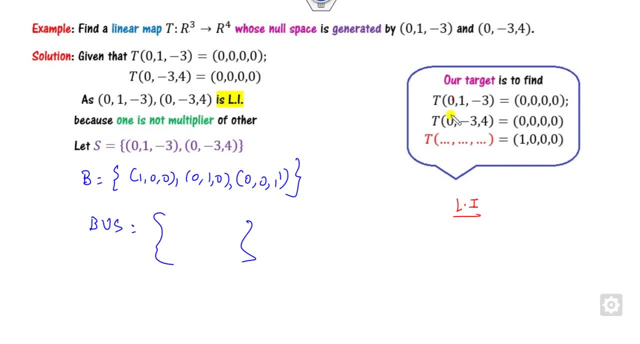 they are linearly independent. clearly say, these two elements are 0, so if i write as a 1, then what is the meaning of that? that means this: this first element is not the scalar multiple of the this. this element is also not the multiple of the others. how you can find the other element you? 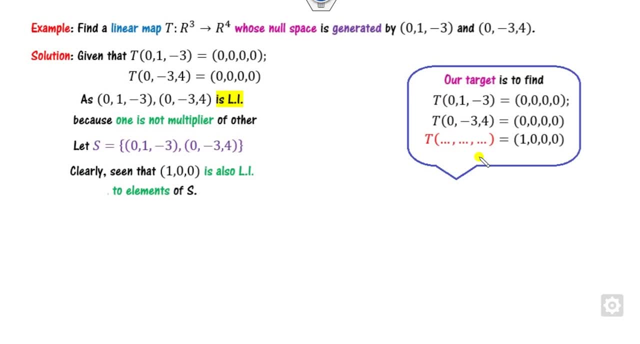 can simply take as a 0. there is no need to write the. any of the elements so clearly says this is also be the ally other. otherwise, this is the first method. otherwise you can write as a. in the previous example, you can write as a matrix and then convert into the echelon form. now, since this value is my here, so you can. 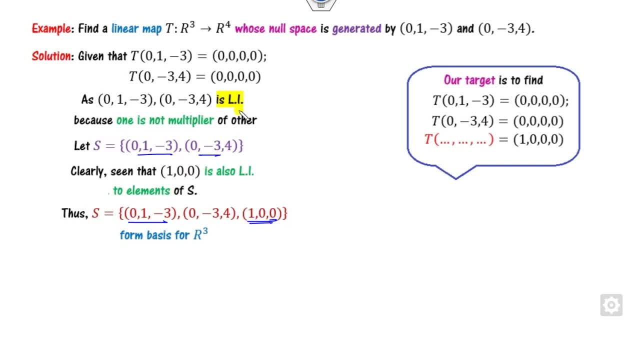 write this as these two values and of this it means your target is to find. these two values are already be there. the first value i can consider as this: the elements of the r4 i can write. rest of the part are similar. you can take the any of the elements from the domain right. value this: you. 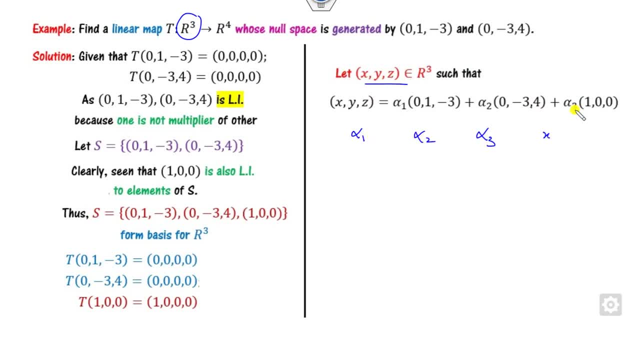 can find the value of the alpha 1, alpha 2 and the other elements from the domain and write the value of this value and alpha 3 in terms of x, y, z. now you can equate them. you can see this is here. after solving these two value, you will get this. take the transformation on the both side, this value. 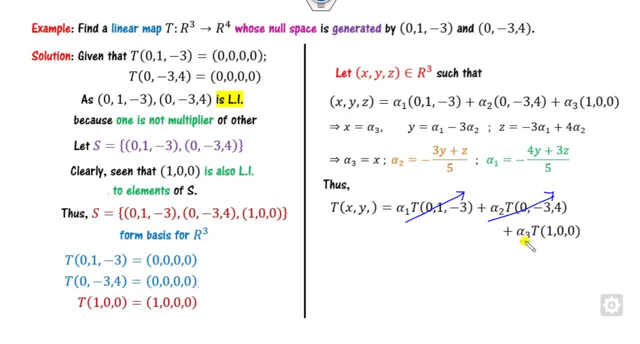 becomes a 0, this value becomes a 0. so only the alpha 3. alpha 3 is my x. i can substitute here as a x. the value of this is my 1 comma 0 comma 0. so this is my linear transformation. so this is the. 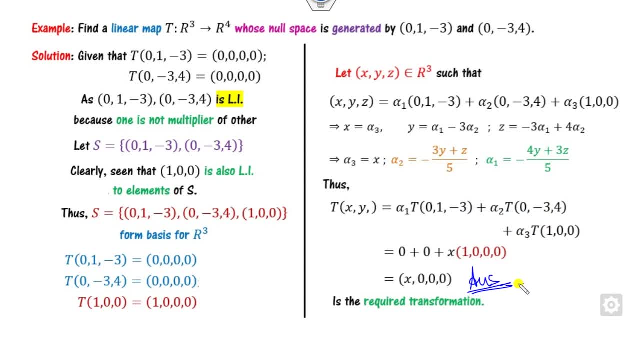 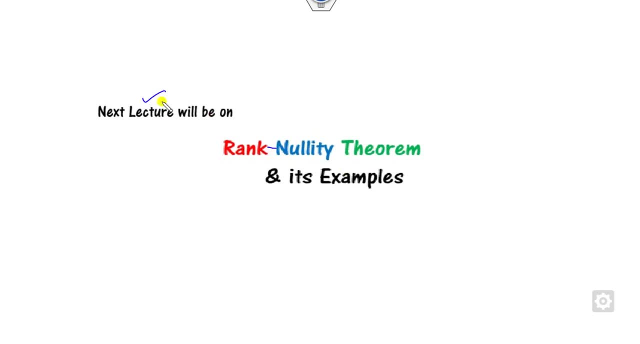 way you can solve the kernel of the linear transformation we will see based on this kernel and this rank space. we will see then rank multi theorem and its example in our next class. till then, you can simply follow this link for finding the various videos. best of luck, students, happy learning.